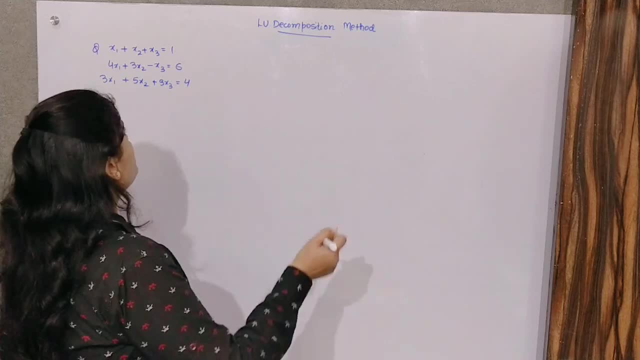 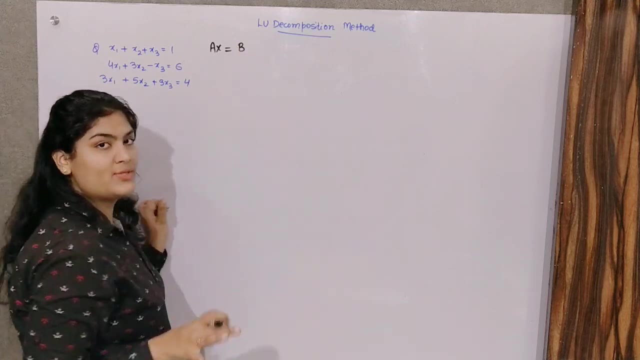 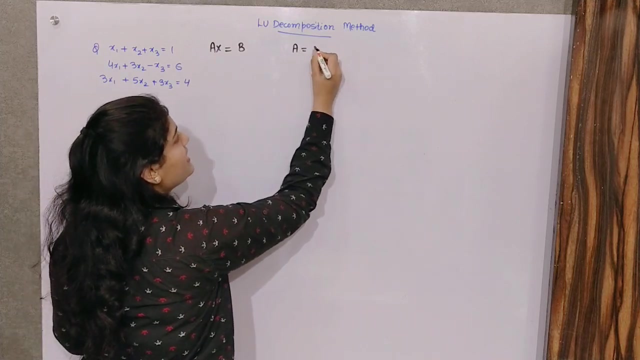 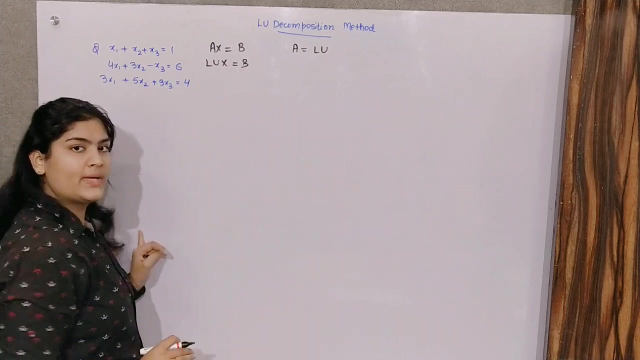 is x1, x2 and x3.. So what you need to do, you know, when we do by matrix inversion method, we have to take: ax is equals to b, right? This is as similar as that. The only difference is you have to split a matrix into L and U, Alright, And then substitute the value of a here, Okay. So let's begin it So: a. you know, the matrix is. 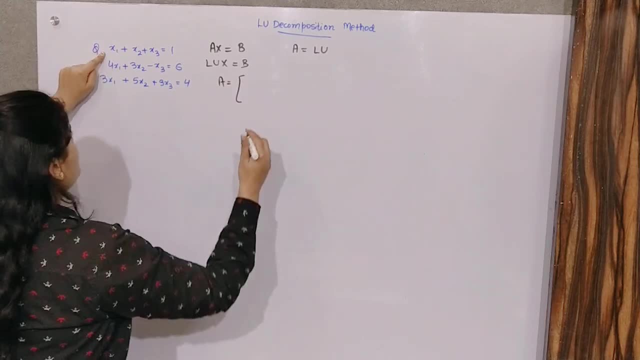 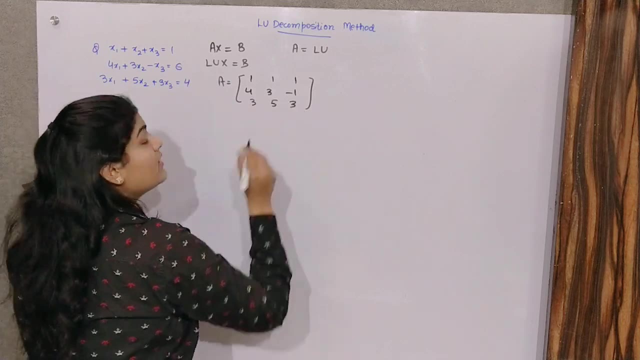 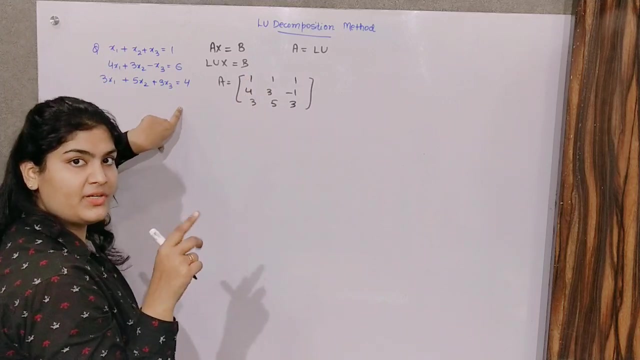 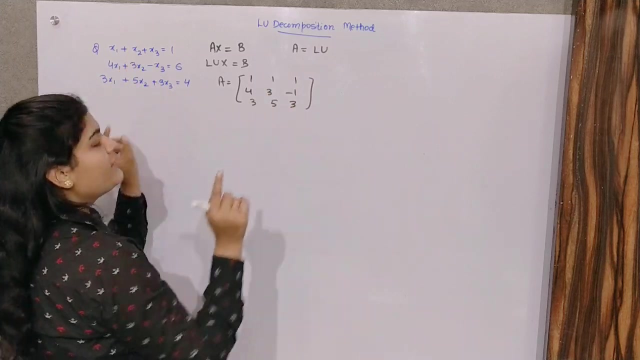 is the coefficient of variables, So 1, 1, 1, 4, 3, minus 1, 3, 5, 3.. Make sure you are taking the right order. The coefficient of x1 here. if any of the coefficient is missing, that means you have to take the value as 0. So the coefficient of x2 here and coefficient of x3 here. Sometimes questions mess up with the order, So you have to. 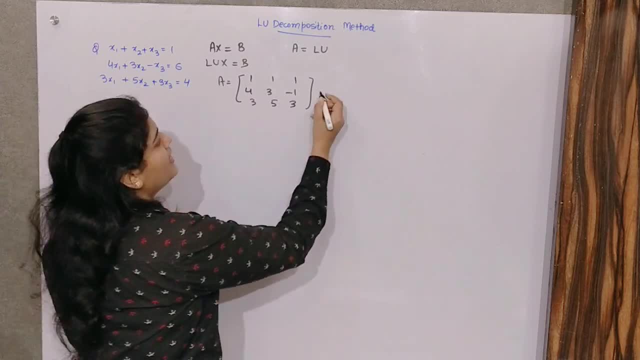 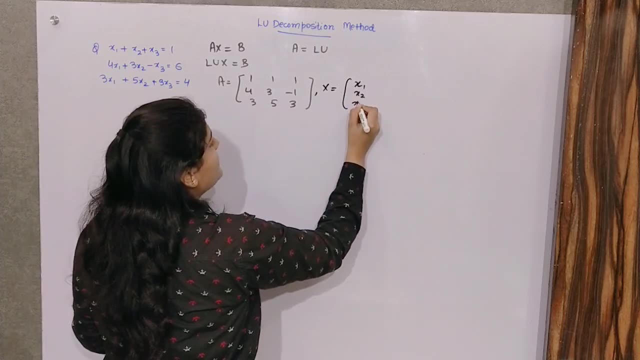 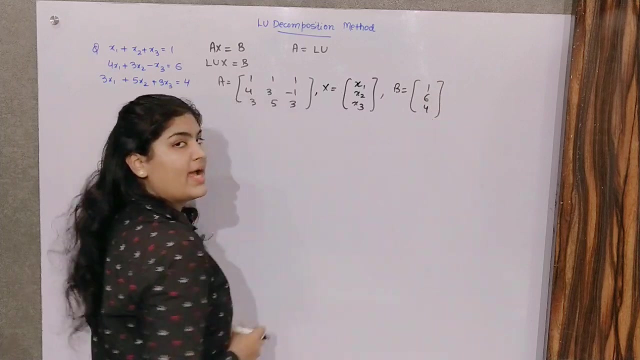 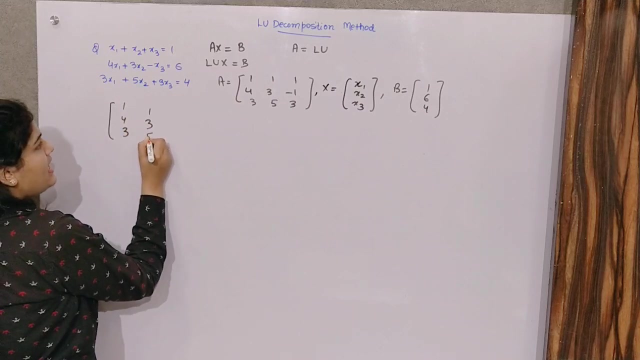 make sure that order is right. So this is a. your x is what? The values for which you have to find out. So x1, x2, x3.. And what is b? You're right inside 164.. Alright, So a is Lu. So let me tell you what is L and what is U. Your L is lower division, lower division. 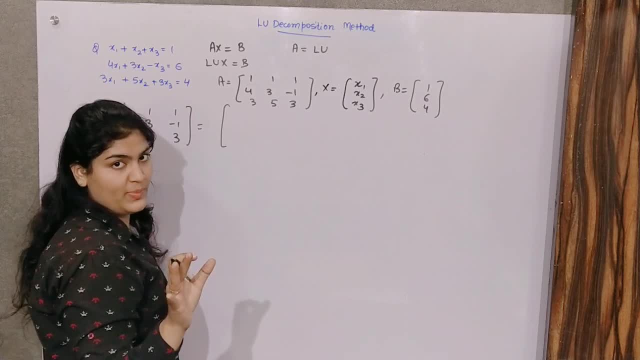 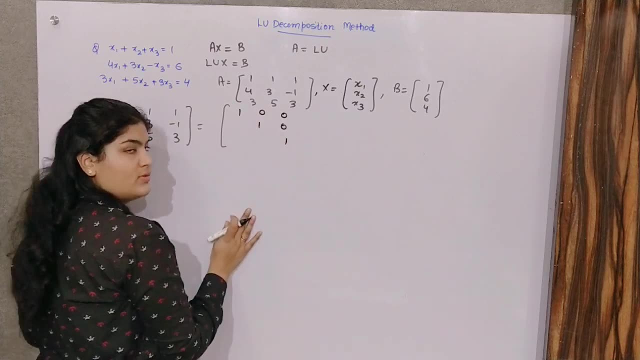 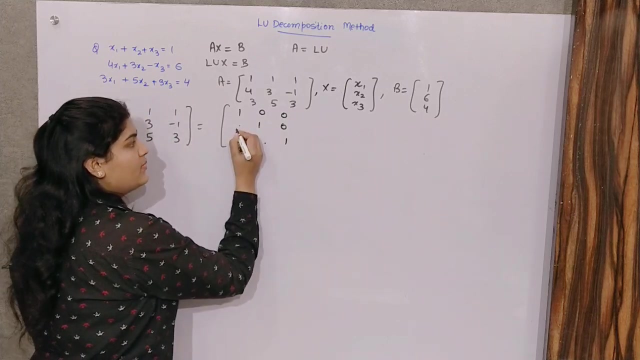 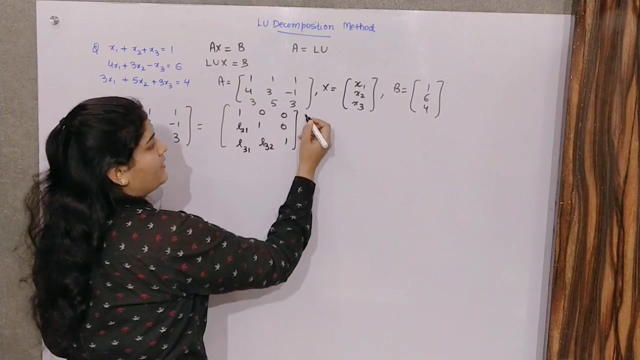 Lower triangular matrix. that means upper triangle would be 0.. The elements of upper triangle would be 0.. So 1, 1, 1 and these are 0s. Now, these 3 terms you have to fill. So you know what is it. 2nd row, 1st column. So this is 2, 1.. 3rd row, 1st column: 3, 1 and 3, 2.. Okay, Then your U 4U. Because it is upper triangular matrix, you have to take the value as 0.. 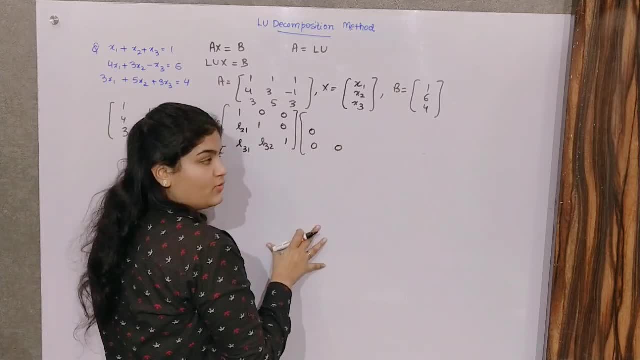 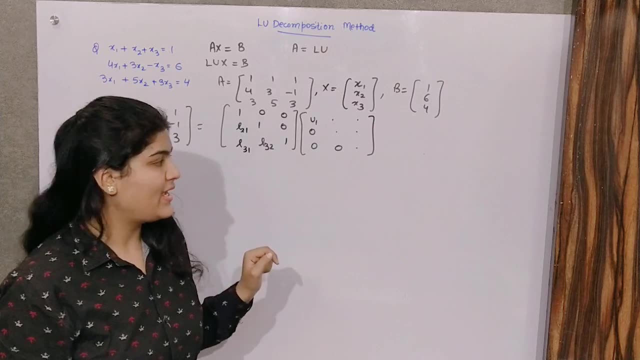 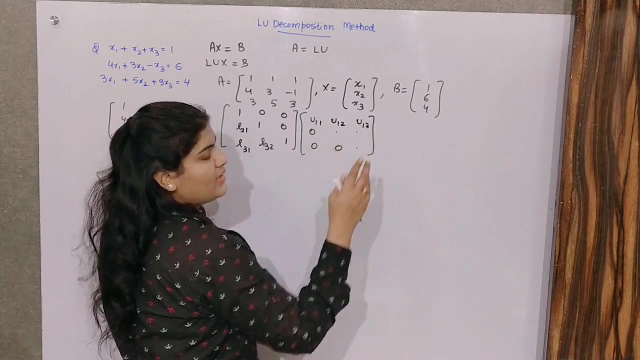 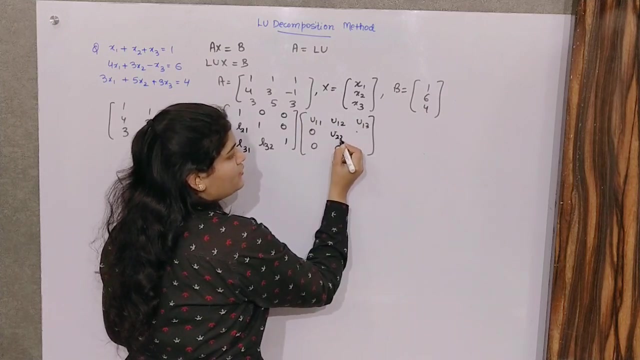 So you have to take lower triangle as 0.. Rest of the element. this is 1st row, 1st column, Because these are the places where you have to put your elements in. So U 1, 1.. U 1, 2.. U 1, 3.. This 1, 1, 1, 2 signifies its position: U 1st row, 1st column. 1st row, 2nd column. 1st row, 3rd column. Then U 2, 2.. U 2, 3. And U 3, 3.. Right. 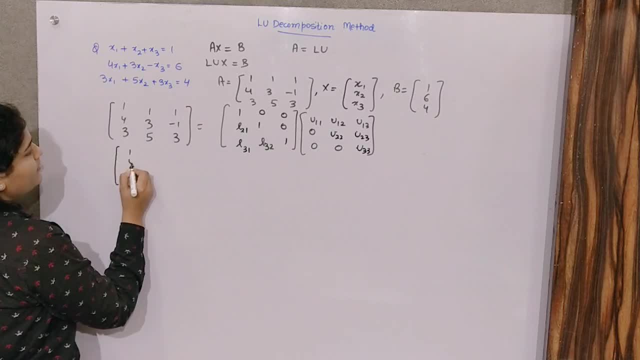 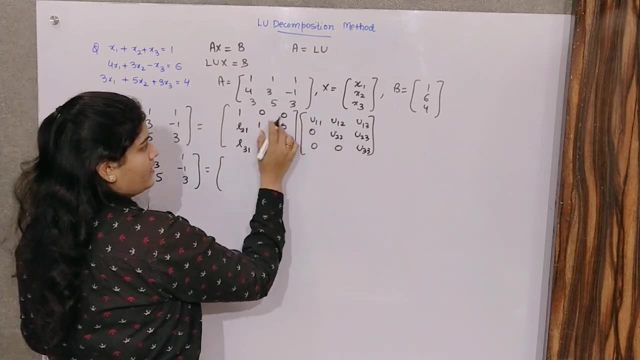 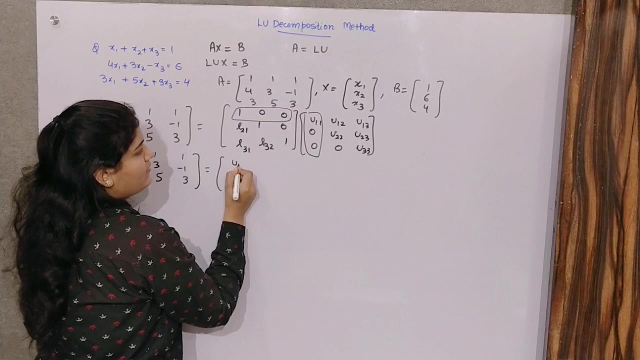 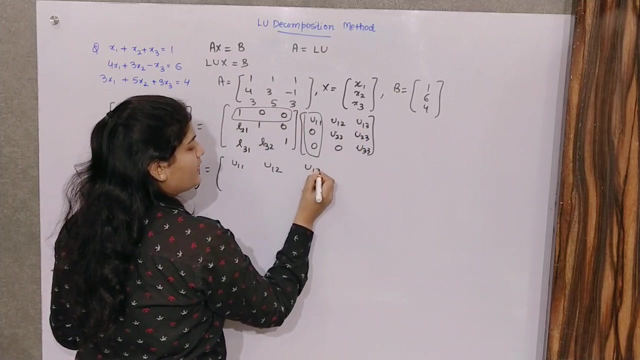 And for all these values, this is all. okay. Multiply 1st row C, 1st row, with 1st column, What is it? This would be multiplied with this, So U 1, 1.. Rest of the element becomes 0.. Then U 1, 2.. 1st row, 3rd column: U 1, 3.. Right, 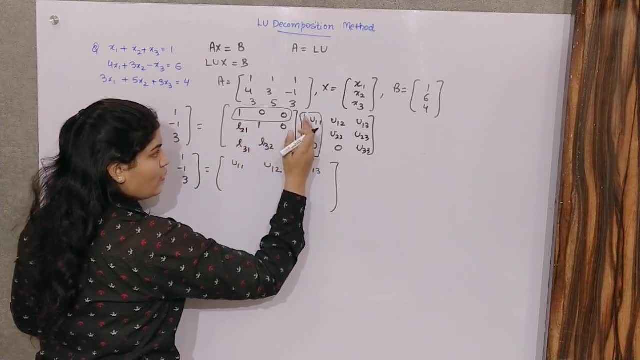 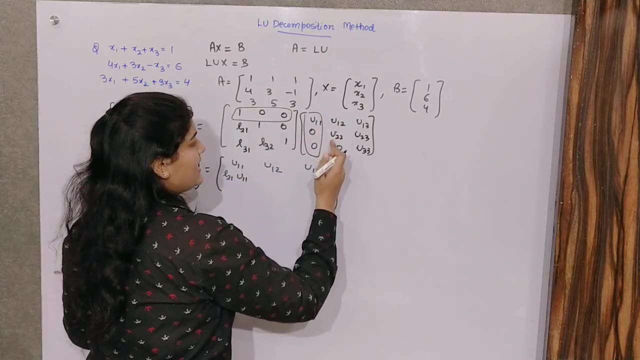 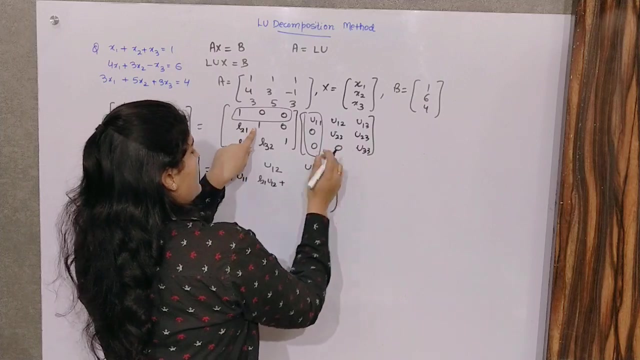 Then 2nd row, 1st column, So C. 2nd row, 1st column would be L 2, 1.. U 1, 1.. Right 2nd row, 2nd column, So L 2, 1.. U 1, 2.. 2nd row, 2nd column, Then U 2, 2.. And this would become 0.. 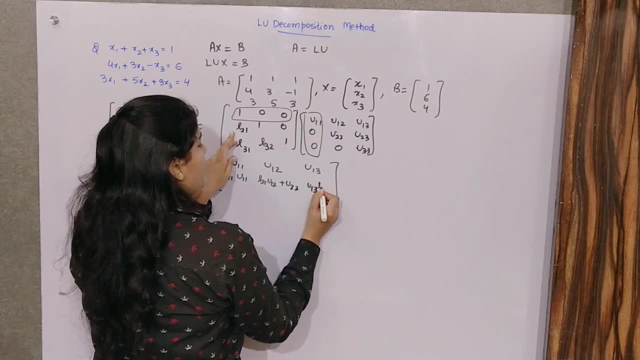 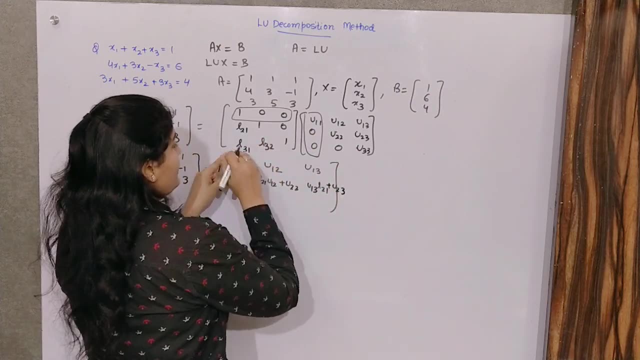 Then 2nd row, 3rd column: U 1, 3.. L 2, 1.. Then this U 2, 3.. And this would become 0.. Then, 3rd row, 1st column. 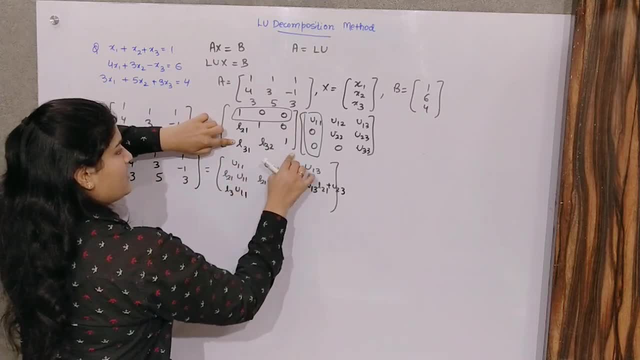 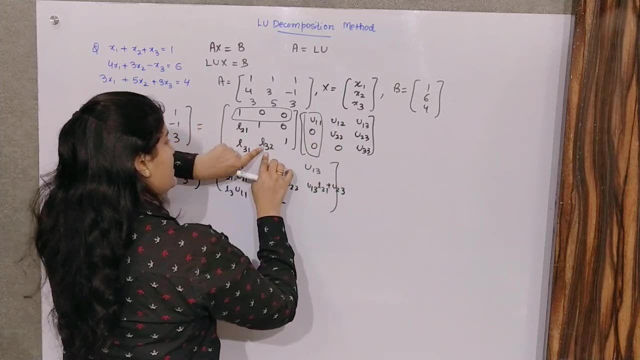 L 3, 1.. U 1, 1.. This would become 0.. 3rd row, 2nd column: L 3, 1.. U 1, 2.. Plus L 3, 2. U 2, 2.. This would become 0.. 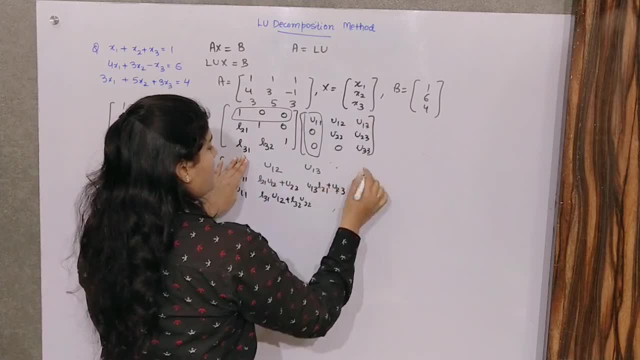 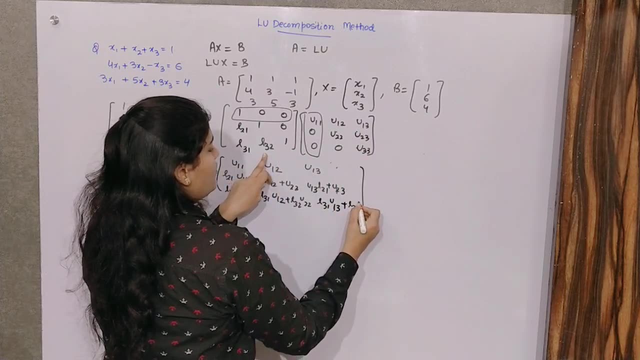 Then 3rd row, 3rd column, So L 3, 1. U 1, 3. Plus L 3, 2. U 2, 3. Plus U 3, 3.. 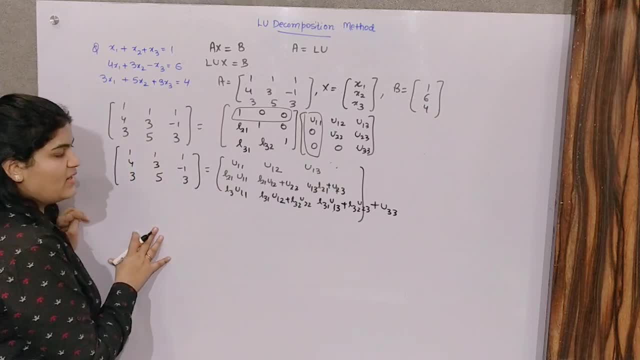 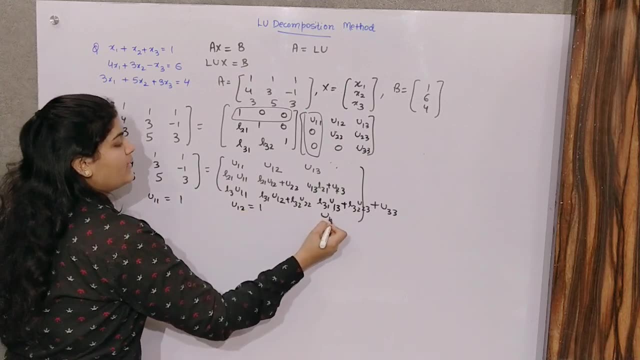 Right Now compare all of the elements with their respective positions. So U 1, 1 is 1.. U 1, 2 is 1.. U 1, 3 is 1.. Right Now here, L 2, 1.. 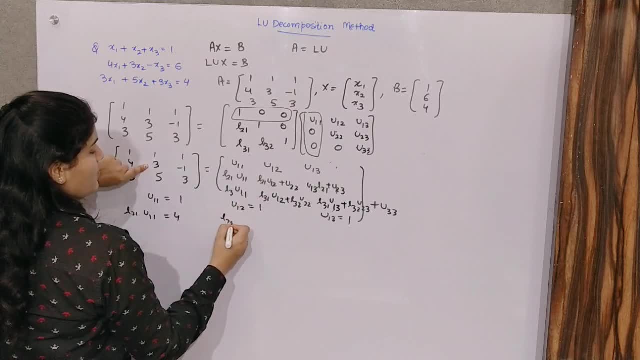 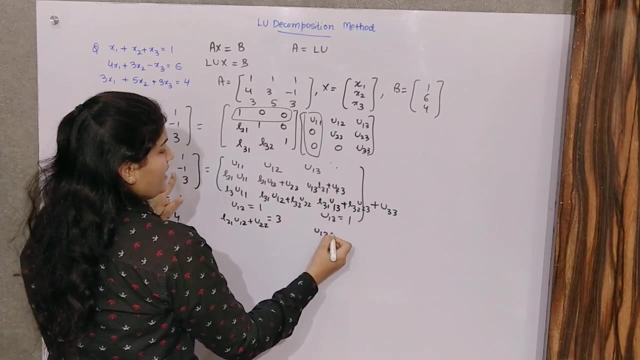 U 1, 1 is 4. L 2,, 1. U 1, 2.. Plus U 2 is U 2,, 2 is 3. U 1, 3.. 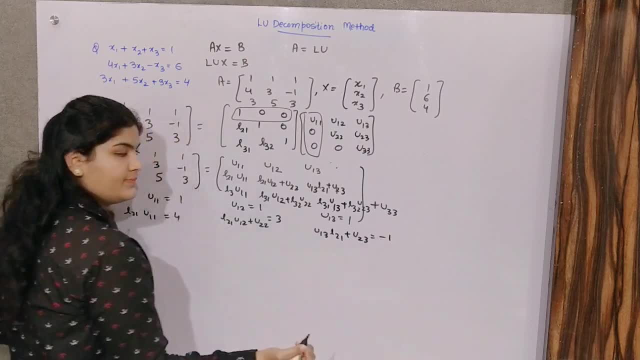 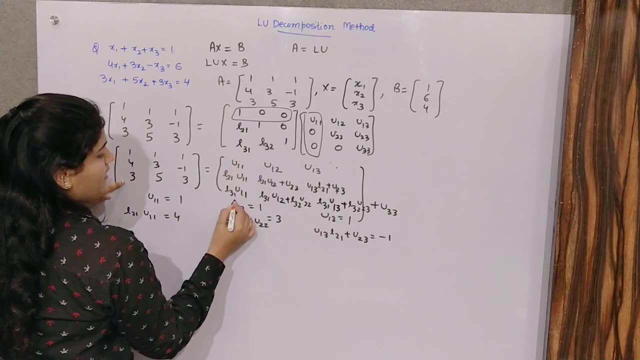 L 2, 1.. Plus U 2, 3 is Minus 1.. Okay, And then L 3.. This is L 3, 1.. Right, So L 3, 1.. 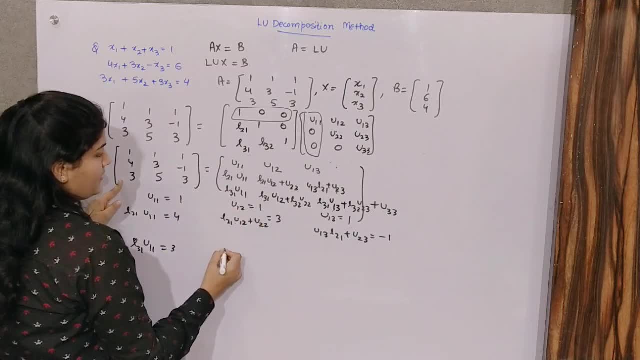 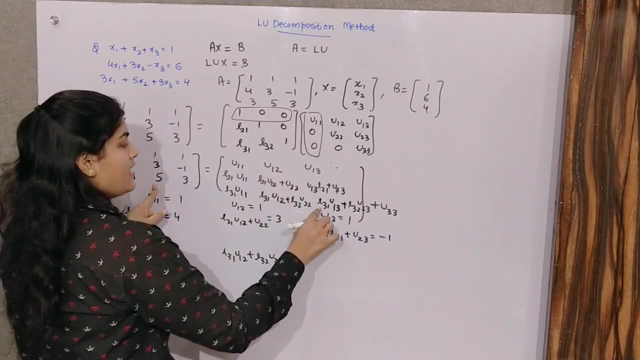 U 1, 1 is 3.. L 3, 1.. U 1, 2. Plus L 3, 2.. U 2, 2 is 5.. Then L 3, 1.. 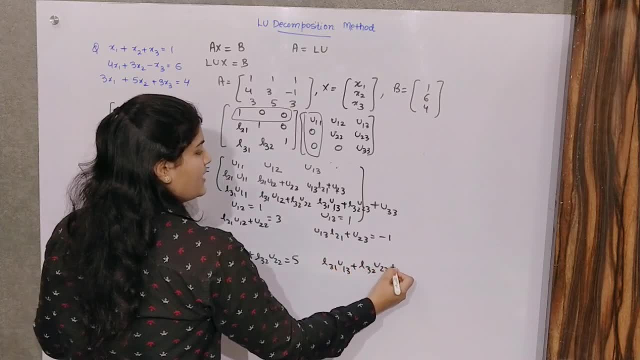 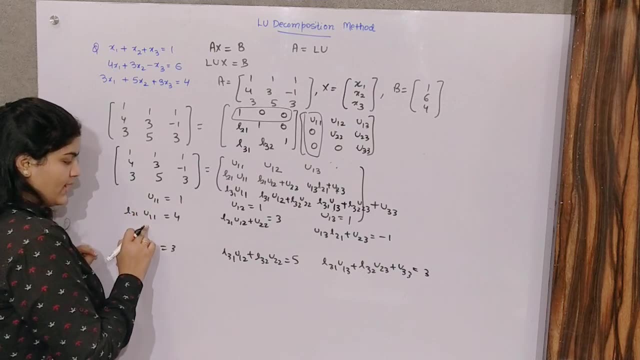 U 1, 3.. L 3, 2. U 2, 3.. Plus U 3,, 3 is 3.. Now get all the values for these values. So U 1, 1 is 1.. 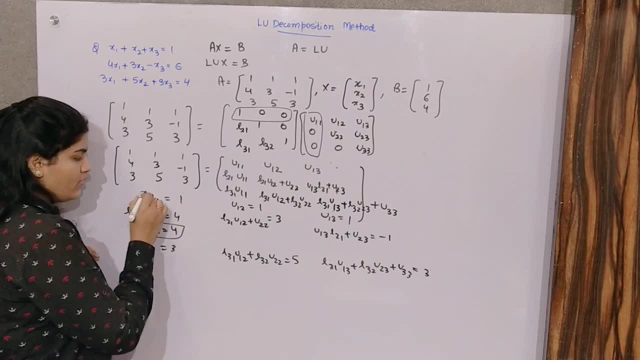 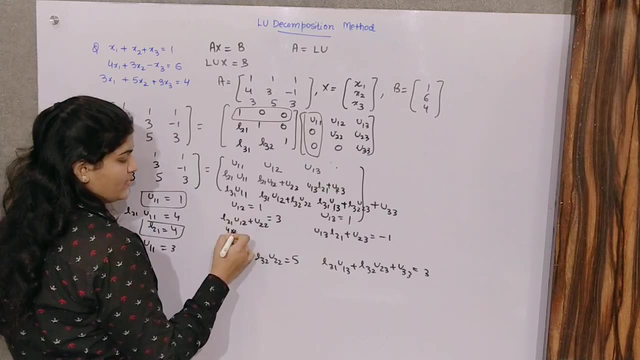 So L 2, 1 becomes 4, divided by 1 is 4.. Alright, Now L 2, 1 is 4.. U 1, 2 is 1.. So U 2, 2 becomes. 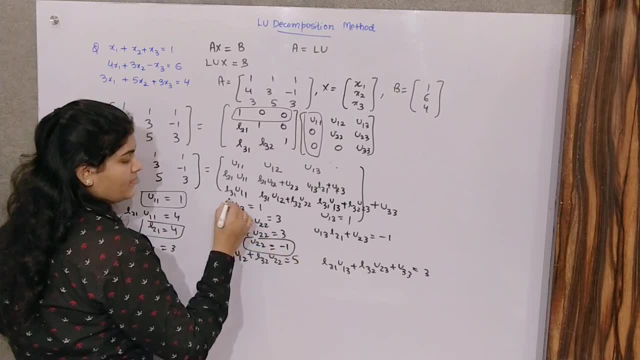 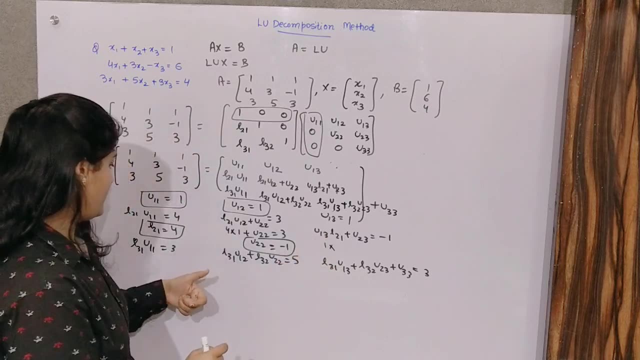 4 times 1 is 4.. 3 minus 4 is minus 1.. Right Then: U 1, 3 is 1.. L 2, 1.. Let's find out the value of here. 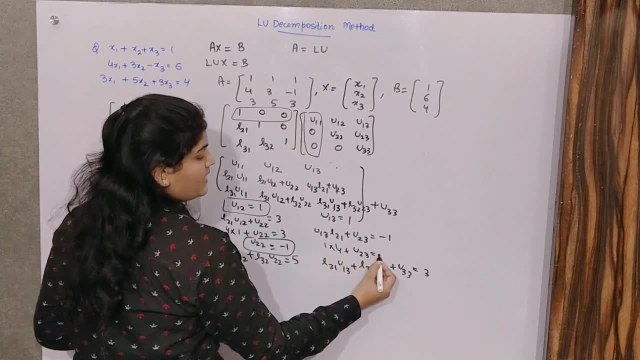 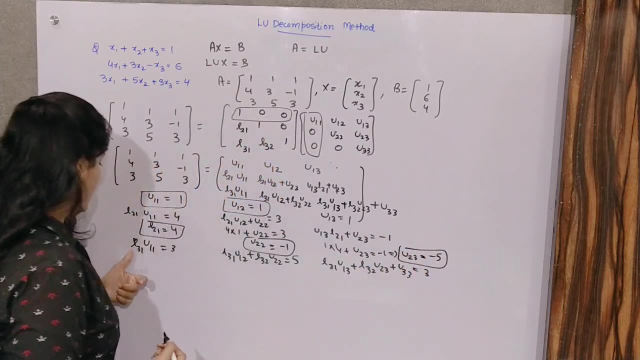 L 2, 1 is 4.. U 2, 3 is minus 1.. So U 2, 3 becomes Minus 1 minus 4 is Minus 5. Now U 1, 1 is 1.. 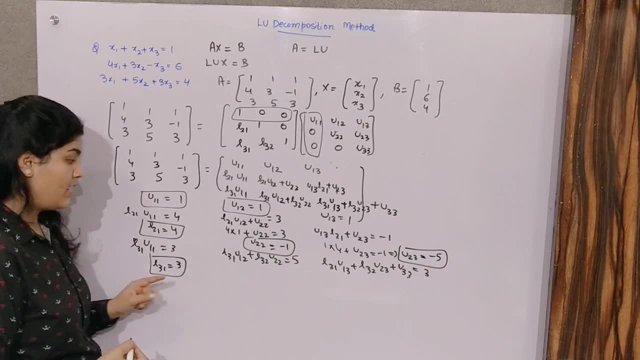 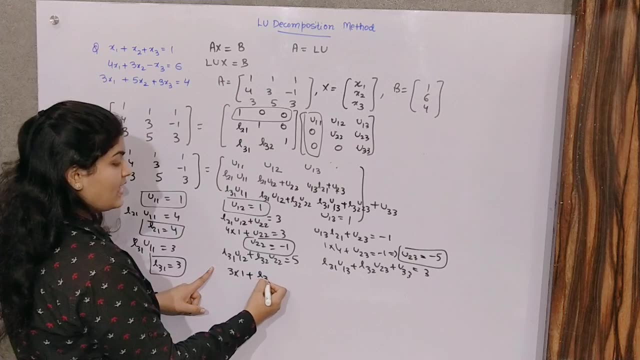 So L 3, 1 becomes 3.. L 3, 1 is 3.. U 1, 2 is 1.. L 3, 2. We have to find out. And U 2, 2 is minus 1.. 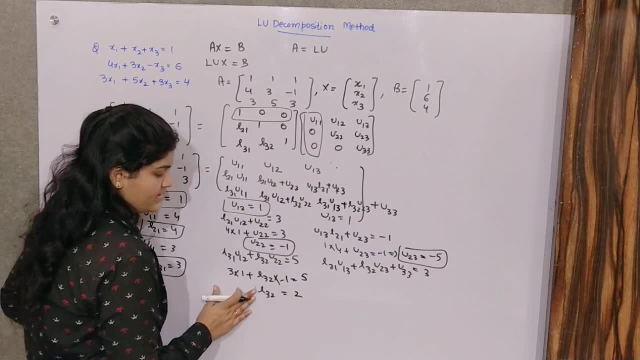 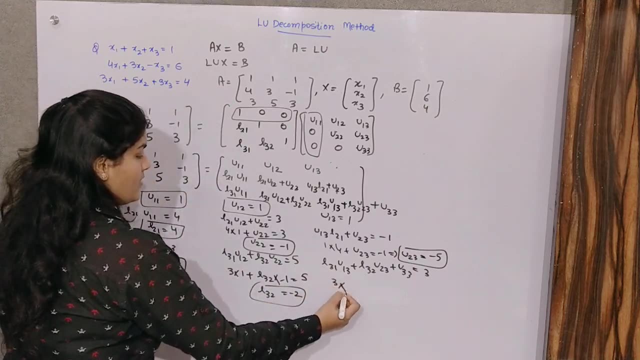 So 5 minus 3 is 2.. And this is here minus 2.. Now L 3, 1 is 3.. U 1, 3 is 1.. L 3, 2 is minus 2.. 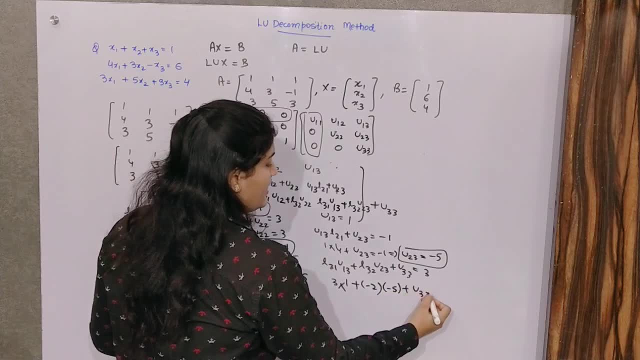 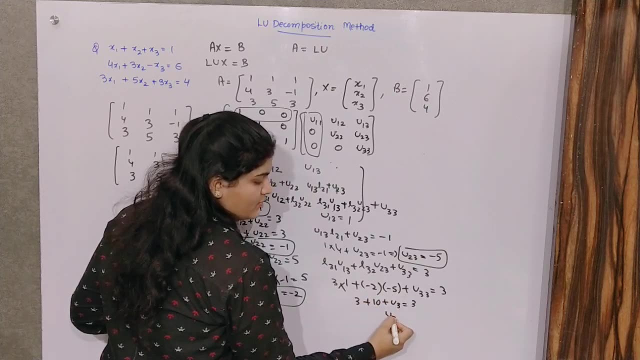 U 2, 3 is minus 5. Plus U 3, 3. 3 times 1 is 3. Minus minus, plus Right, So U 3 becomes 10. That is also minus 10.. 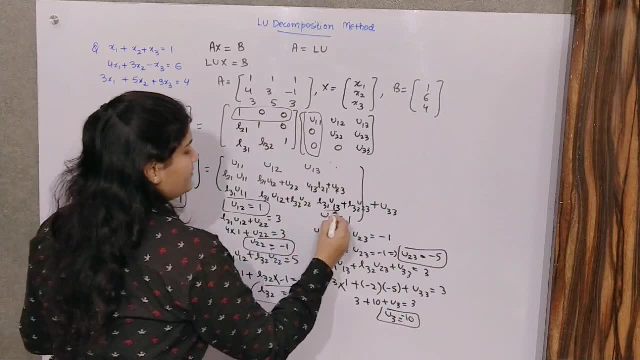 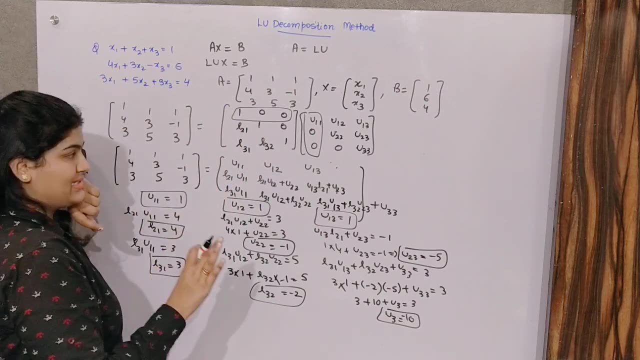 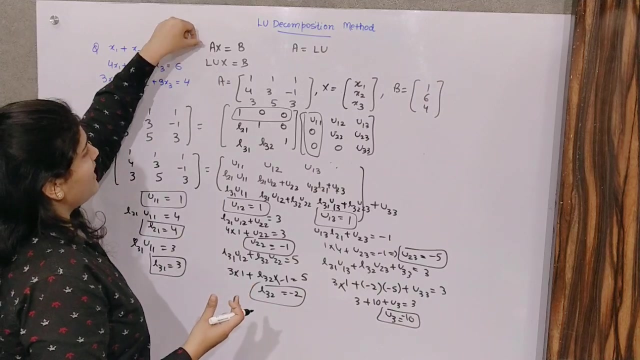 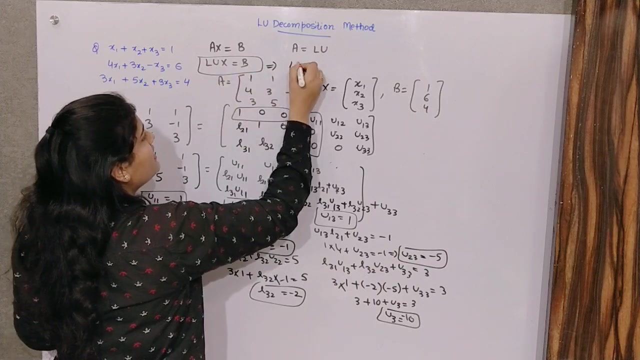 Right. So you have got all these values. Now substitute. So you have got your lower triangular matrix and upper triangular matrix, LU, right, If you substitute or put the value of A as LU in this? And let us suppose that your UX is something called Y. 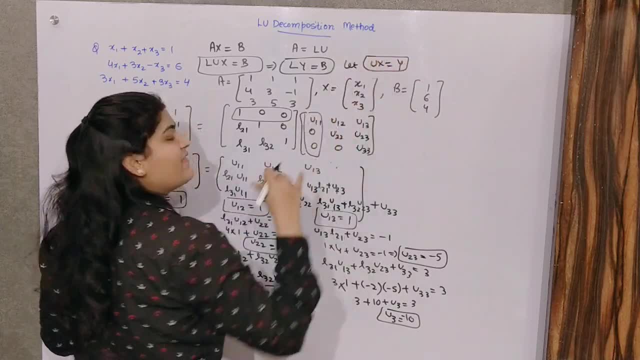 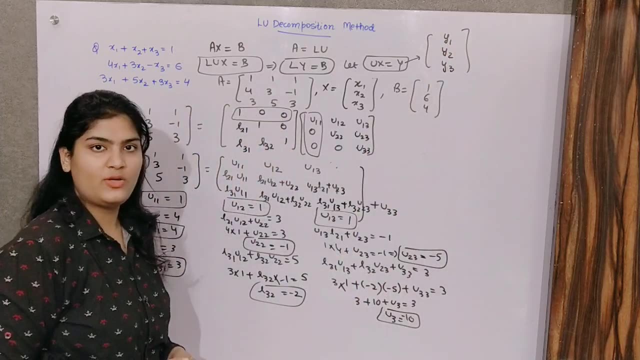 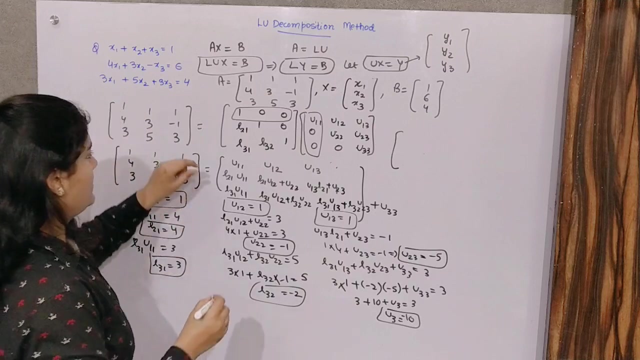 Now let UX is Y, Y, Where Y is a matrix having the elements Y1,, Y2,, Y3.. Okay, So what you have to do, This is U. What is your U? See, this is your U. 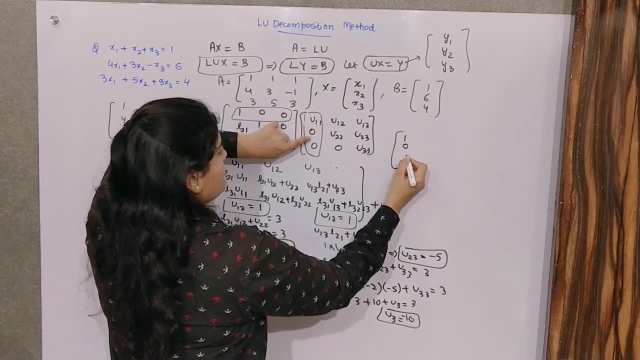 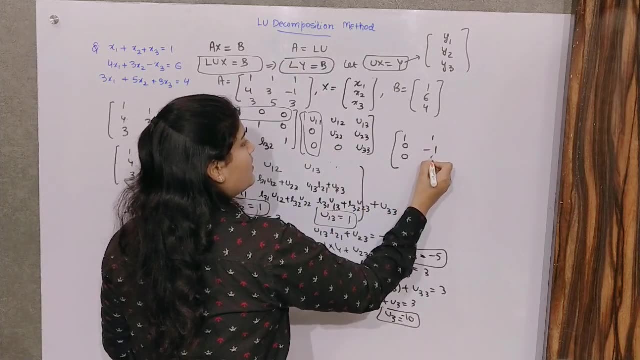 U 1, 1,, which is 1.. 0, 0.. U 1, 2,, which is 1.. U 2, 2 is minus 1.. This is 0.. So U 1, 3 is 1.. 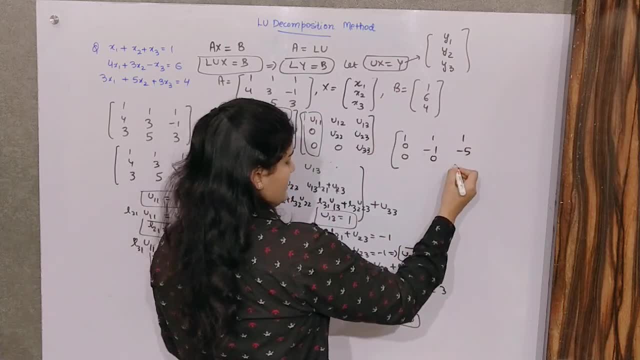 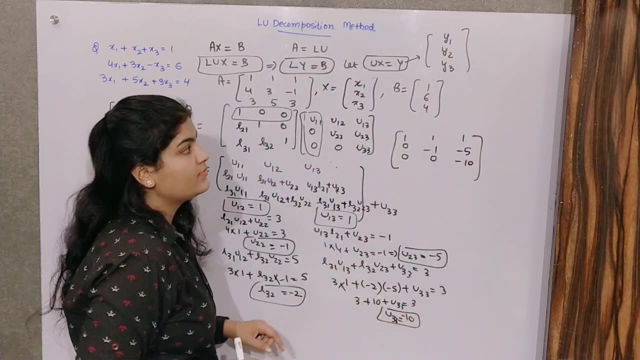 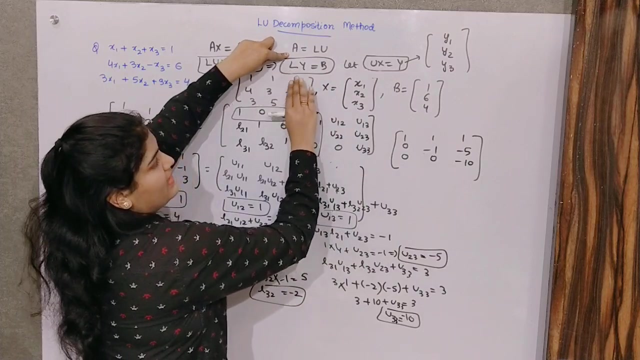 U 2, 3 is minus 5.. And U 3, 3 is minus 10.. This is your U. You have taken your UX as Y right, So now your equation is this: LY equals B right. 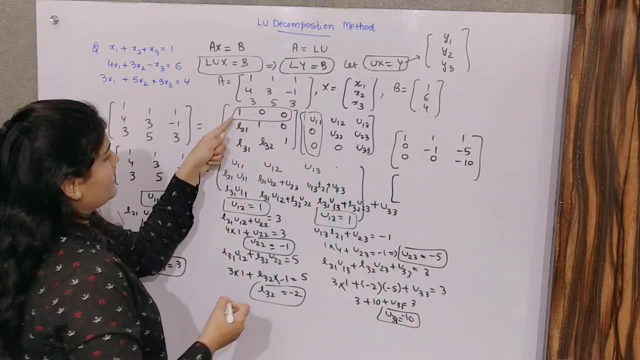 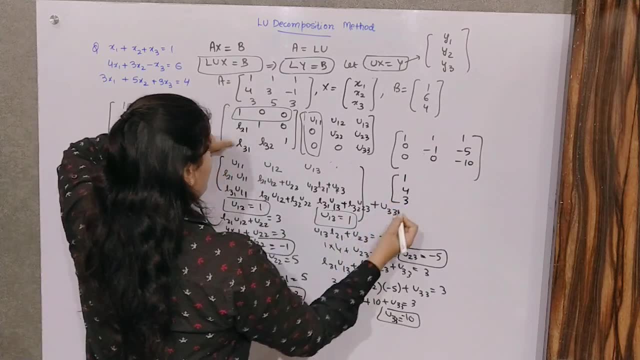 So your L is What is your L? 1. L 2, 1 is 4.. L 3, 1 is 3. 0, 1. L 3, 2 is minus 2.. 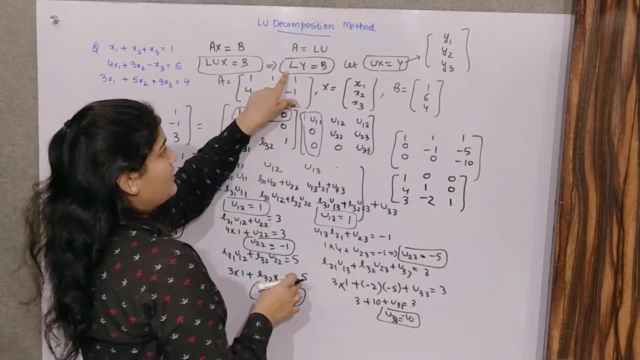 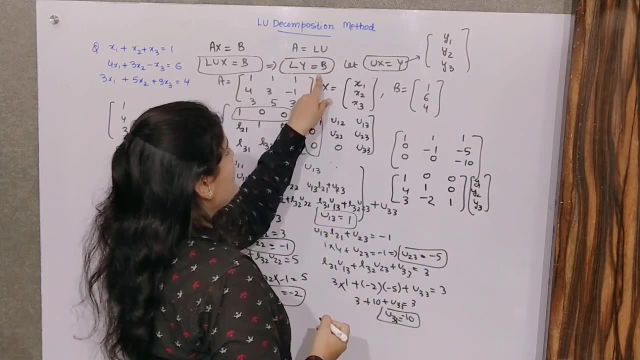 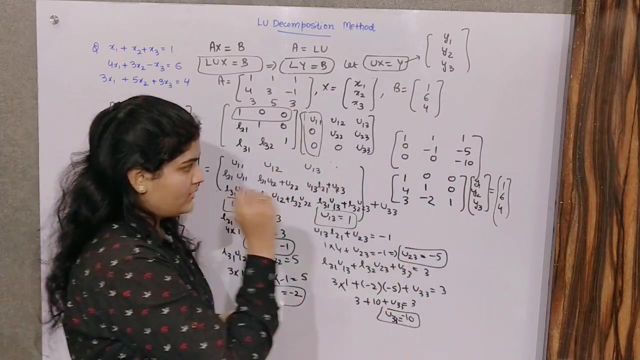 0, 0, 1.. This is your L, Your Y is what Y1, Y2, Y3 is equals to B, which is what 164.. So from here you can find out the value of Y1,, Y2,, Y3. 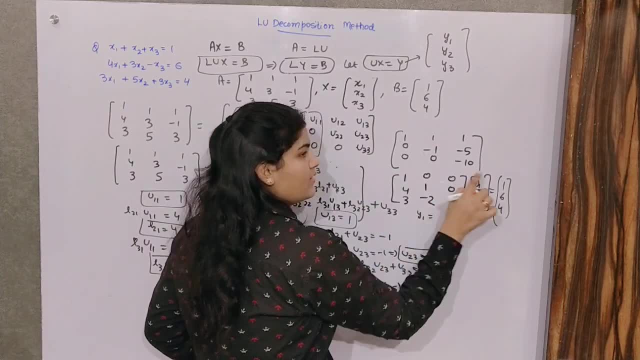 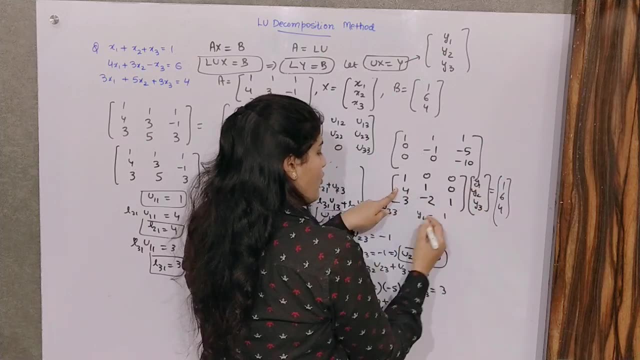 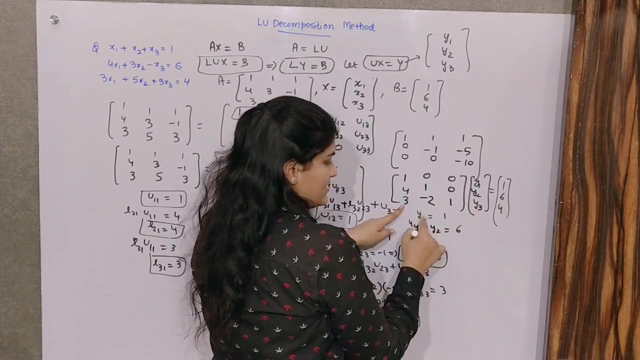 What it would be. First row, first column. So Y1 is 1.. Right See, first row, first column. This is Y1.. This is 4Y1 plus Y2 equals 6.. So your Y1 is what. 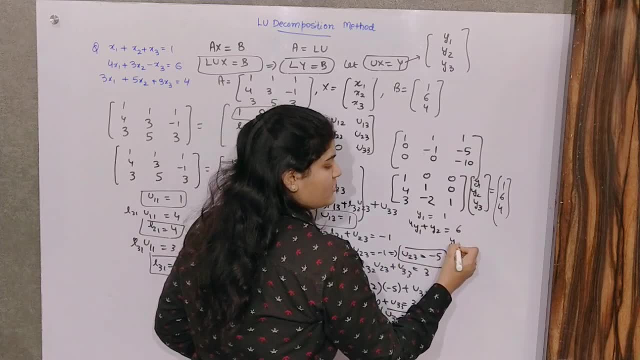 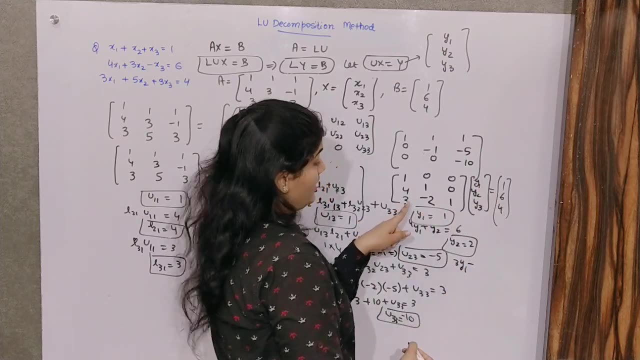 1. 4 times 1 is 4.. 6 minus 4 is 2. Right, And what is your Y3?? So 3Y1 minus 2Y2 plus Y3 equals 4. Right, Right. 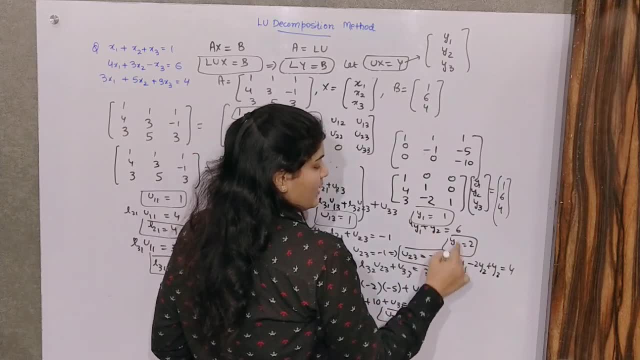 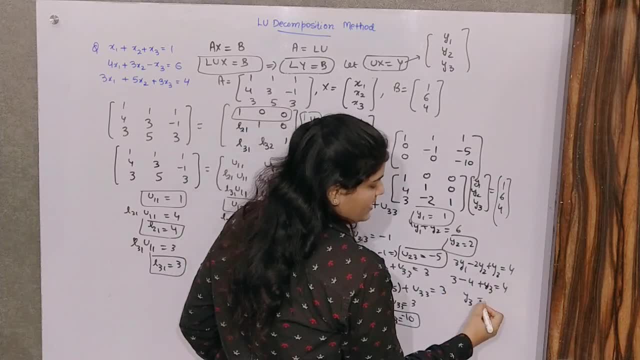 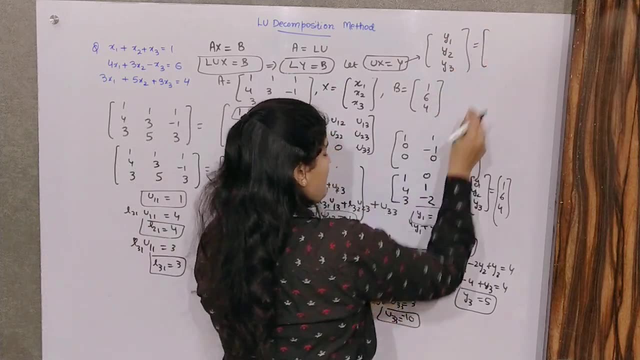 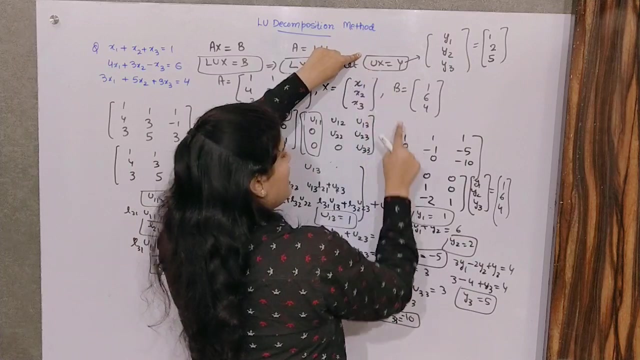 4 minus 3 is minus 1.. 4 plus 1.. Right, You have got your Y matrix. You have got your Y matrix as 1, 2 and 5. Right. So if you substitute here, your value of U is this: 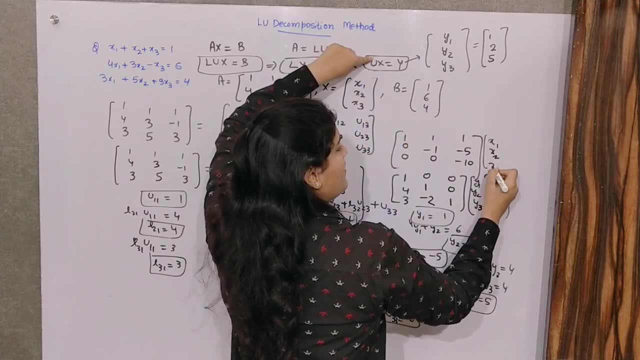 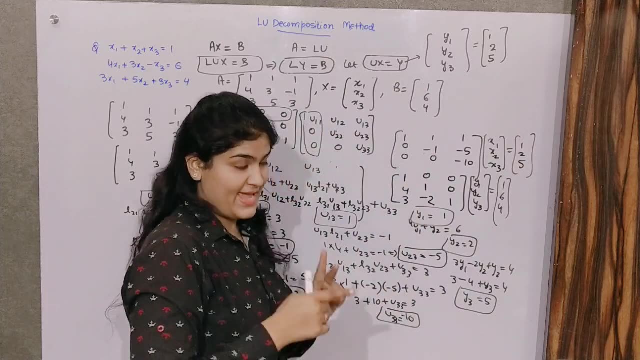 Right. So X is X1,, X2, X3 and Y is what? 1,, 2,, 5.. Now you can find out the value of X1,, X2,, X3. How? Let me solve it here. 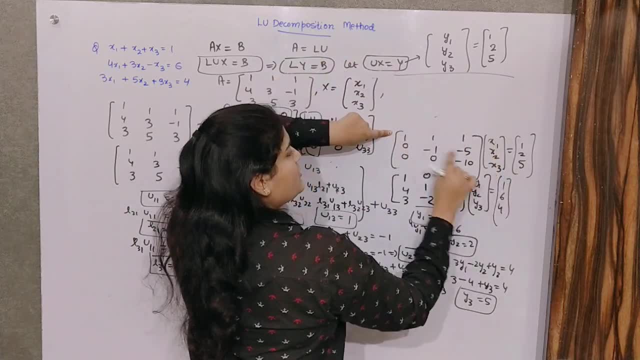 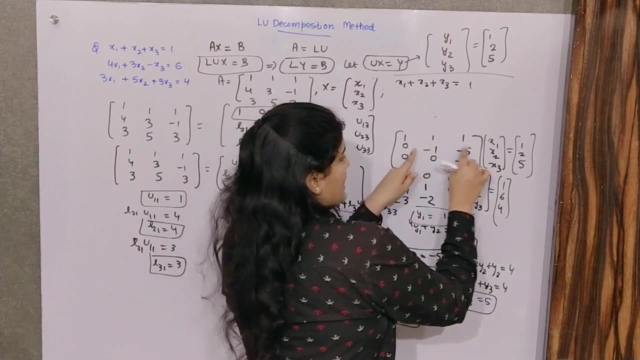 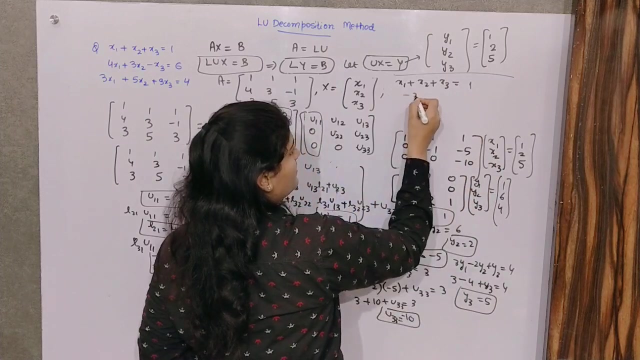 So first row, first column: X1 plus X2 plus X3 equals 1.. Second rows: this is second row, then first column. So 0 times X1 is 1.. So 1 times X1 is 0,. minus 1X2 minus 5X3 equals 2.. 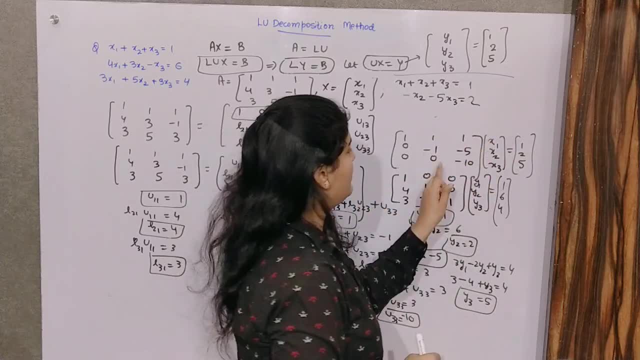 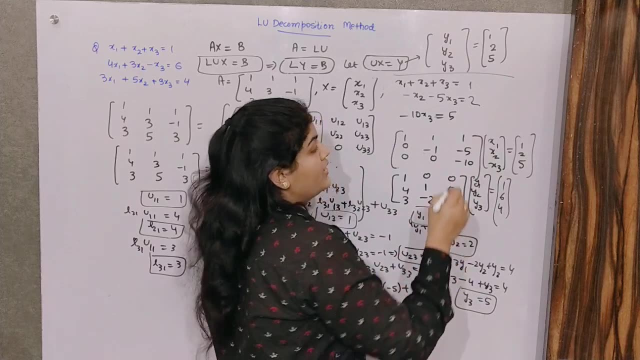 And then third row, then first column: this is 0, this is 0 and this is minus. 10X3 equals 5.. So from here, your X3 is 5 by 10, that means 1 by 2.. 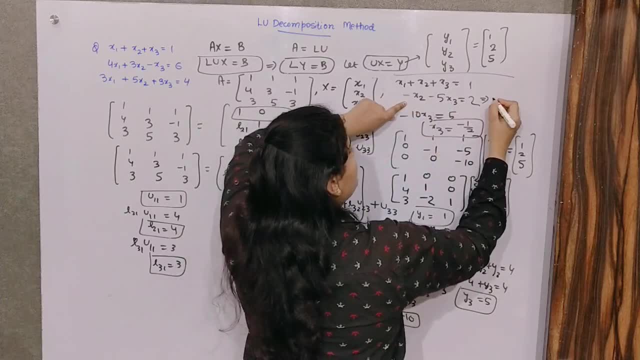 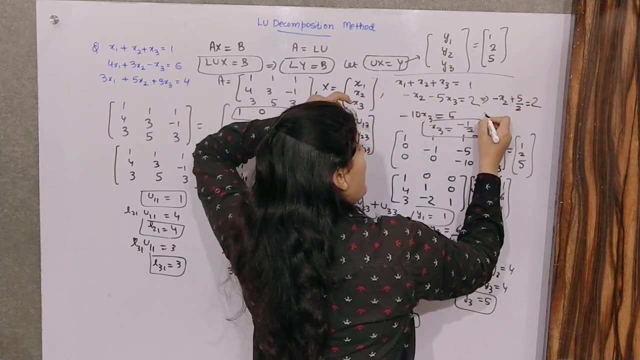 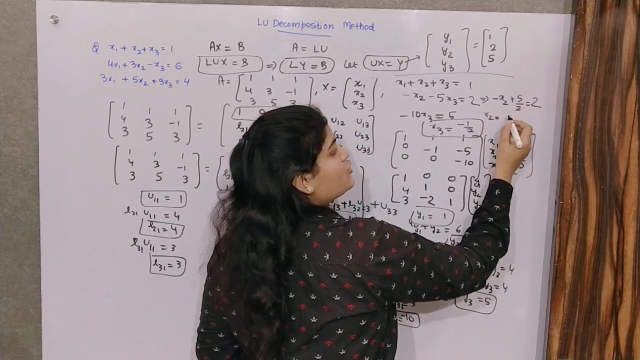 From here your X3 is minus 1 by 2.. So minus minus plus 5 by 2 equals 1.. So your X2 becomes 5 by 2, 3.. Take this X2 to right hand side and bring this 2 onto left hand side. 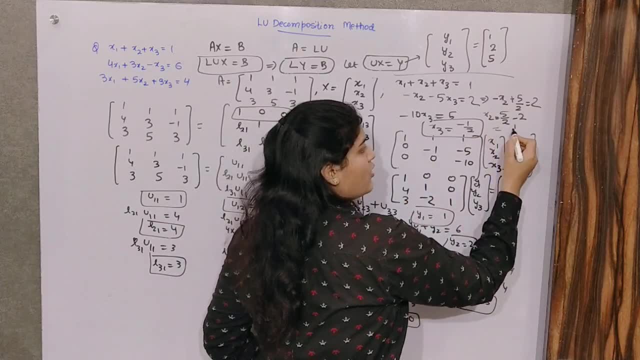 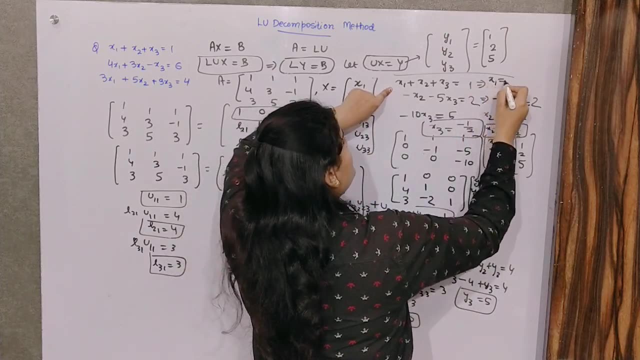 So 2 times 2 is 4, 5 minus 4 is 1.. So your X2 becomes 1 by 2.. Right, And now it comes to X1.. So X1 is 1 minus X2, minus X3.. 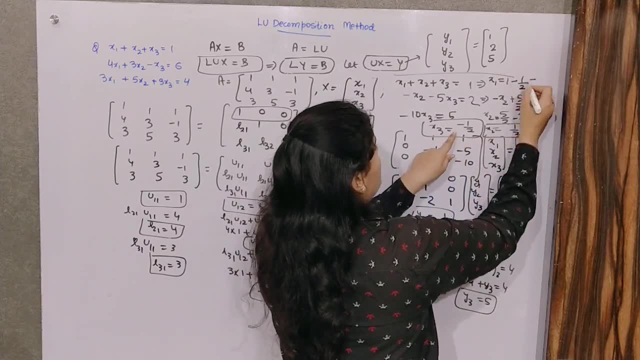 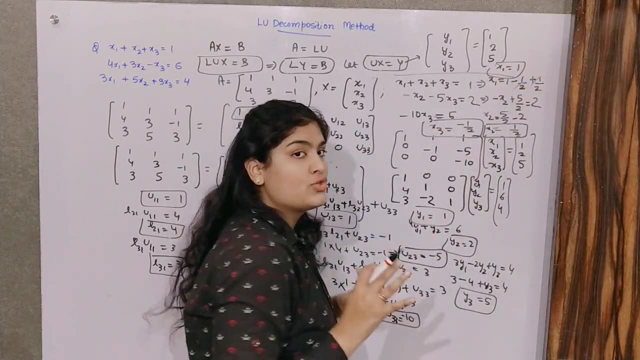 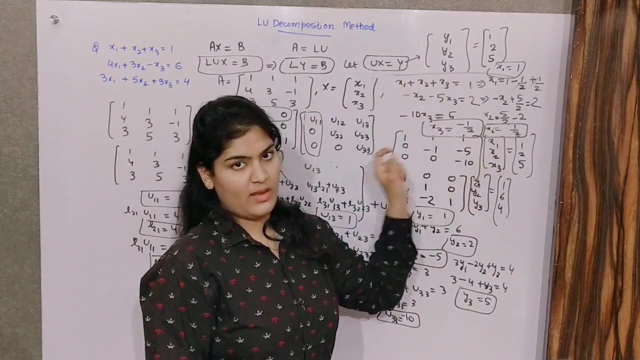 So X2 is 1 by 2 minus X3 minus minus plus. So this is cancelled. What is X 1.. So you can see your values of X1, X2, X3 are 1, 1 by 2 and minus 1 by 2 respectively. 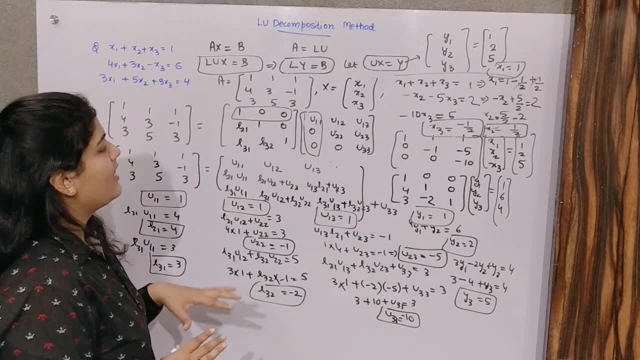 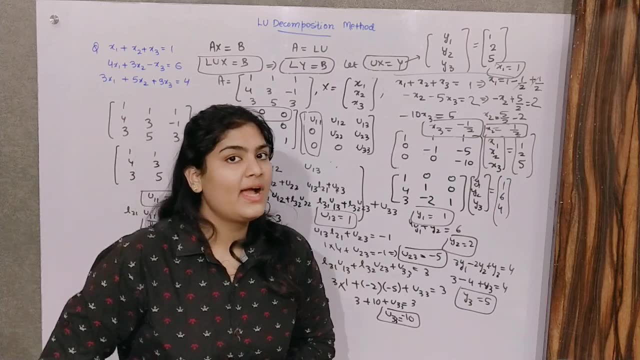 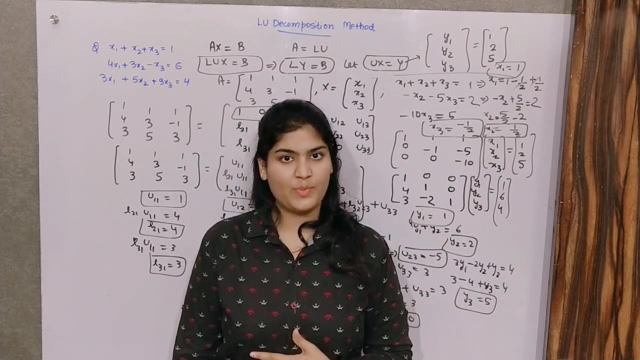 I know you might be thinking of that. okay, with this matrix inversion method, we could have solved it in much easier way. But you know what guys Question has asked specially? this is, I think, the question from 2016 December question. 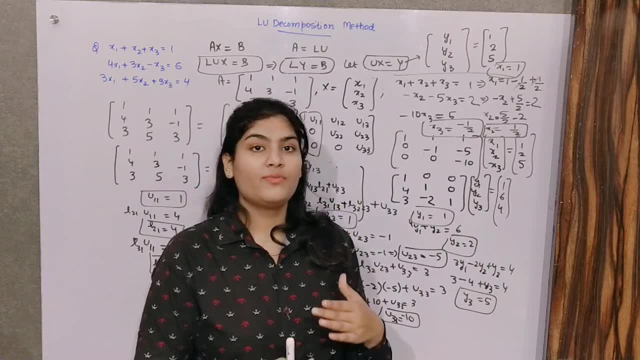 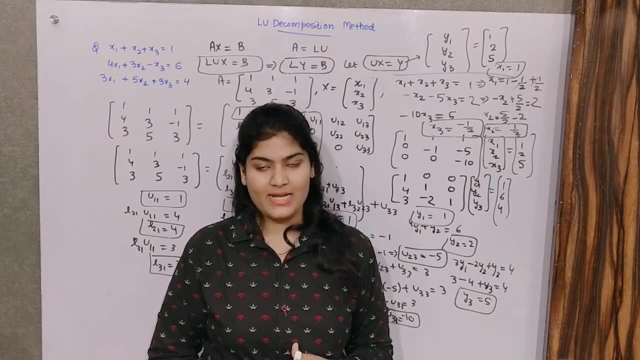 paper of BSE and question has specially asked: solve it via or through LU decomposition method? Then you have to follow what question is asking for right. So that's why you must know how you can find out the value by splitting the matrix. 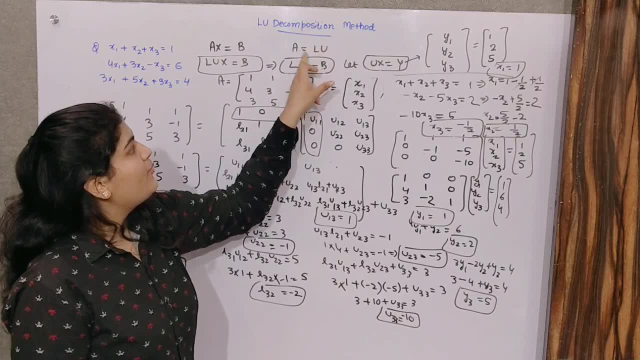 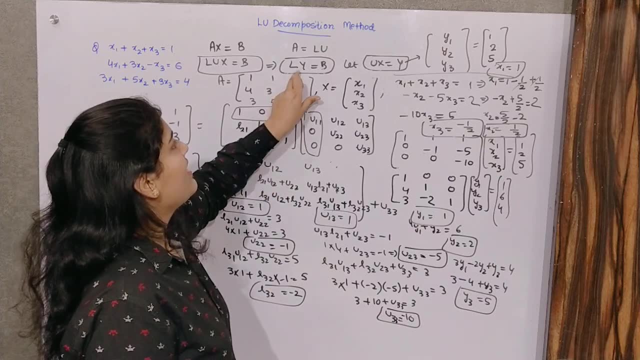 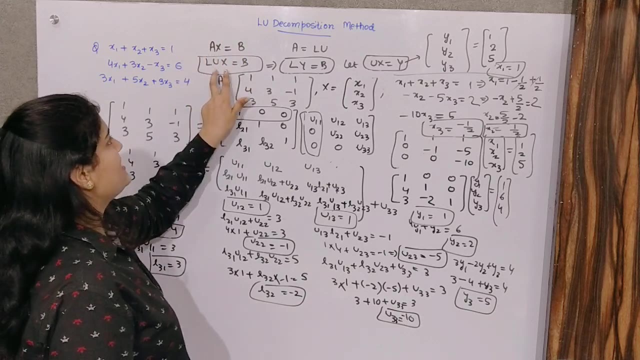 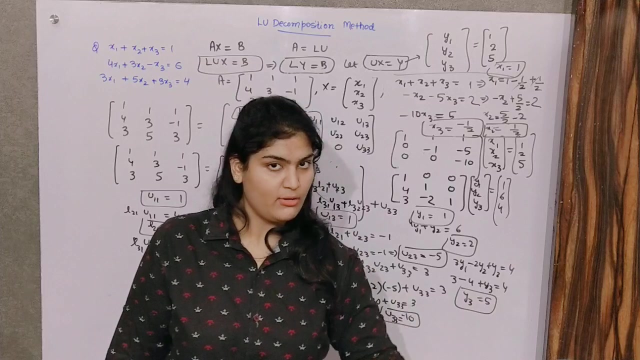 into L and U and then putting it, find out the value of these variables, putting it in these forms and then consider this: AX is equal to B form. put the value of A as LU, consider this as Y, find out the variables of Y and then find, through that, the value of X. 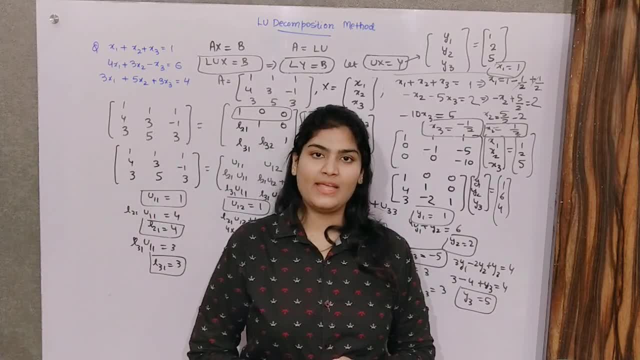 I hope you understand it and if so, then don't forget to like, share and subscribe to my channel. I am really sorry, guys, that I am not monotonous in my job, but I should be. I will definitely try to be more monotonous in my job.